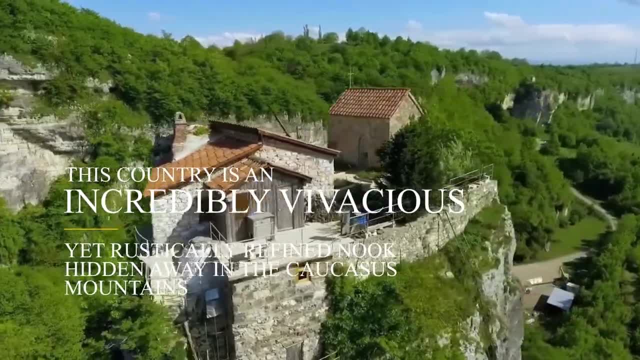 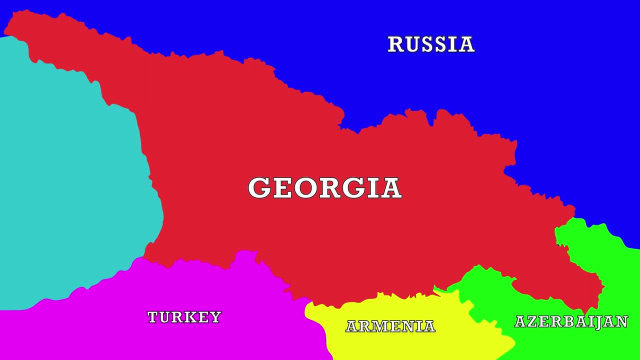 Let's dig into it. This country is an incredibly vivacious yet rustically refined nook hidden away in the Caucasus mountains, bordered by Russia, Turkey and Armenia and Azerbaijan to the north, south and east, and has a coastline along the Black Sea to the west. The total area of the 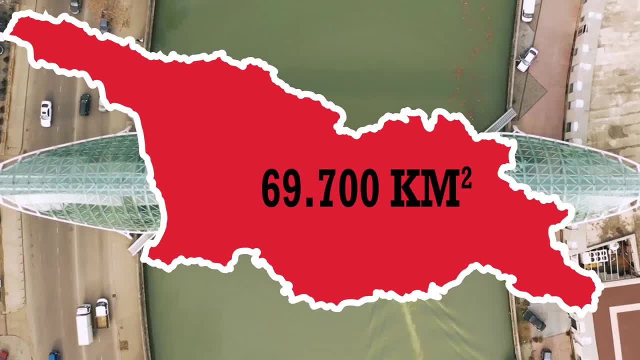 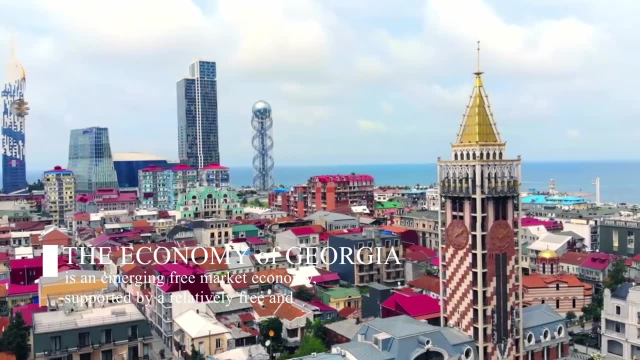 country is 69,000 square kilometers. The population of Georgia is about 3,000, 700 square kilometers, pretty much sandwiched between the greater and lesser Caucasus mountains. The economy of Georgia is an emerging free market economy supported by a relatively free and. 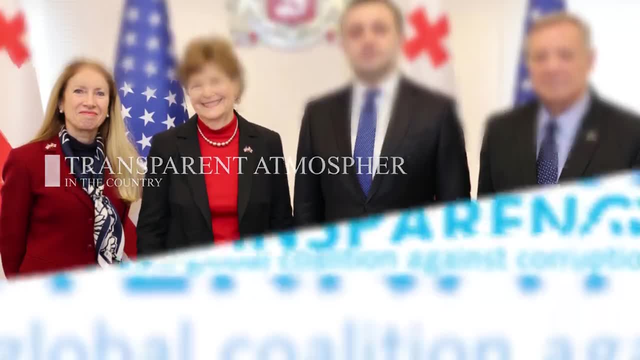 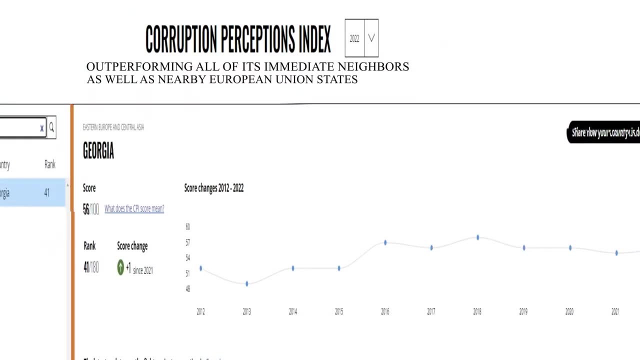 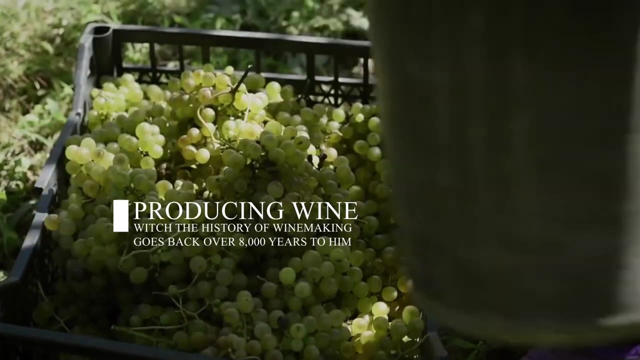 transparent atmosphere in the country. According to latest Transparency International's report, Georgia is the least corrupt nation in the Black Sea region, outperforming all of its immediate neighbors as well as nearby European Union states. Georgia's economy has historically been centered on Black Sea tourism, producing wine, which the history of winemaking goes. 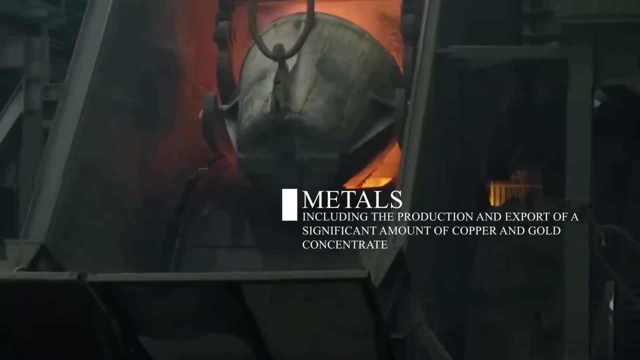 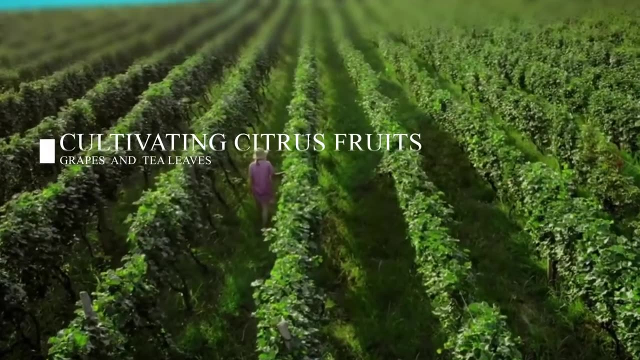 back over 8,000 years to him, metals, including the production and export of a significant amount of copper and gold concentrate, machinery, chemicals and textiles, as well as cultivating citrus fruits, grapes and tea leaves. and, of course, its rich history, culture and natural. 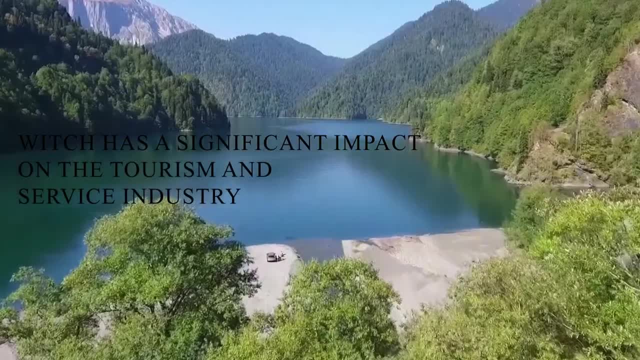 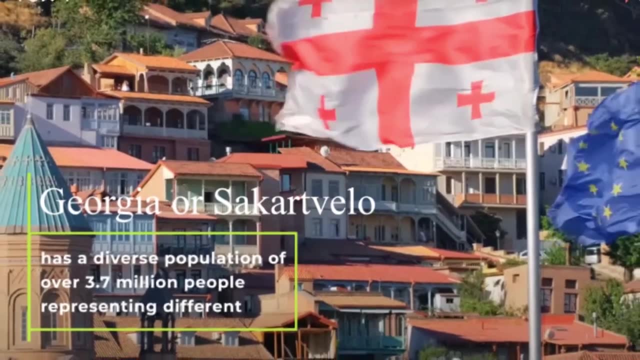 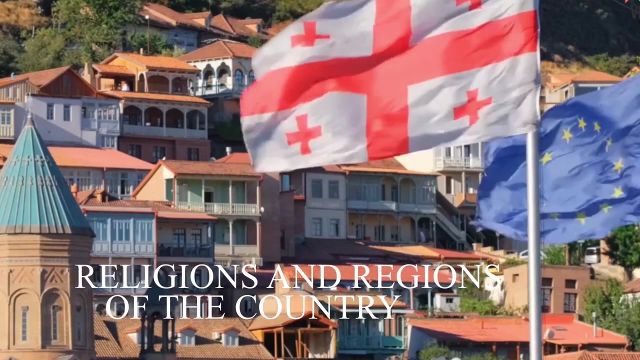 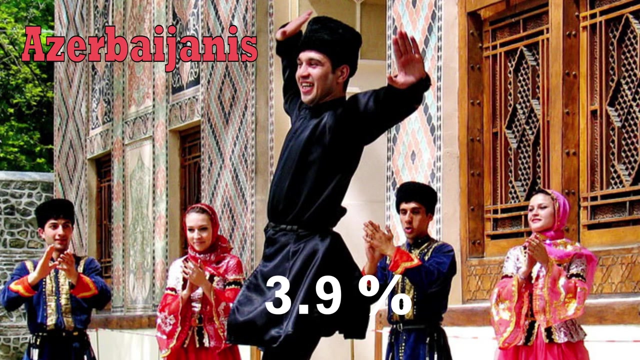 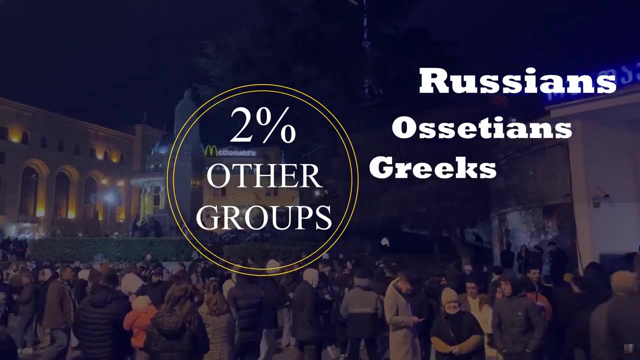 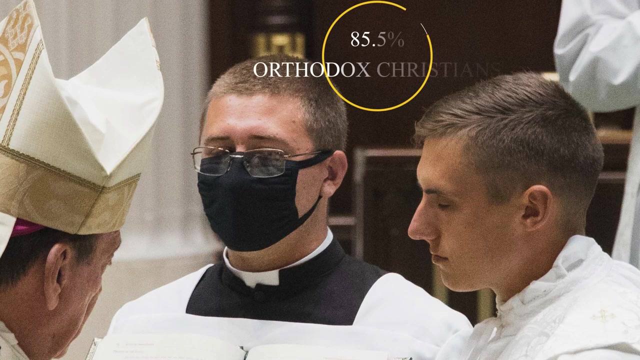 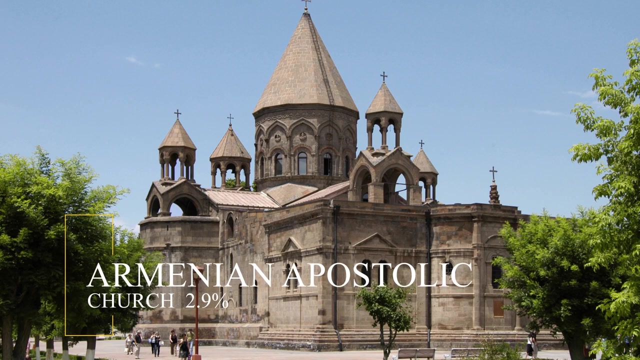 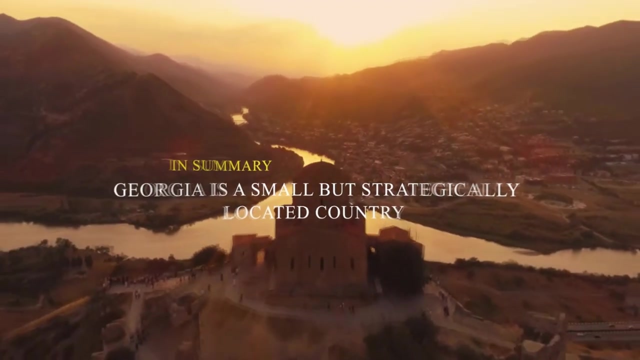 beauty, attracting millions of visitors each year, which has a significant impact on the tourism and service industry and, ultimately, the economy of this country. For more information, visit wwwtransparencyorg. In summary, Georgia is a small but strategically located country with a rich history and culture. 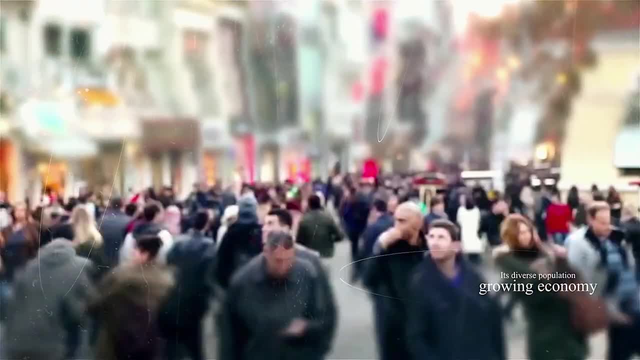 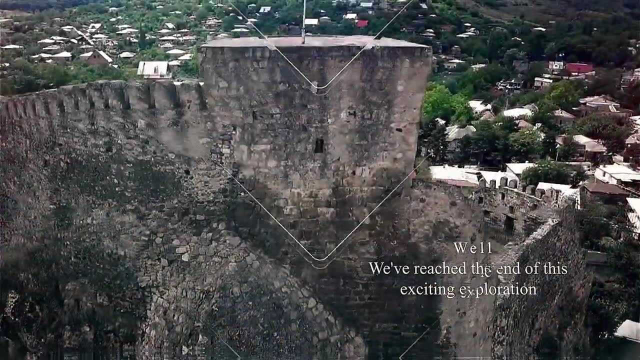 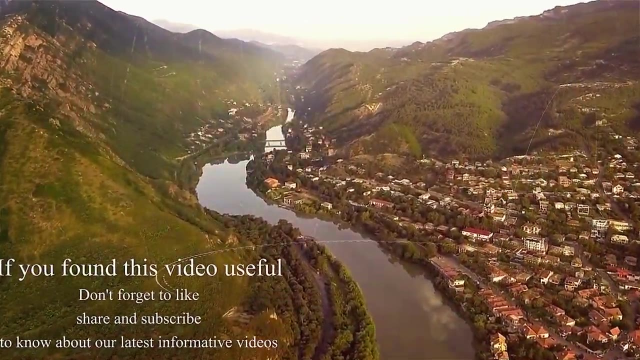 Its diverse population, growing economy and natural beauty make it an attractive destination for everyone planning a safe investment, a comfortable trip or living in a new beautiful country. Well, we've reached the end of this exciting exploration. If you found this video useful, don't forget to like, share and subscribe to know about. our latest informative videos.